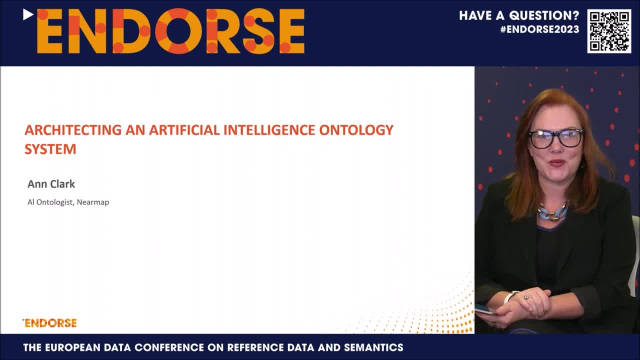 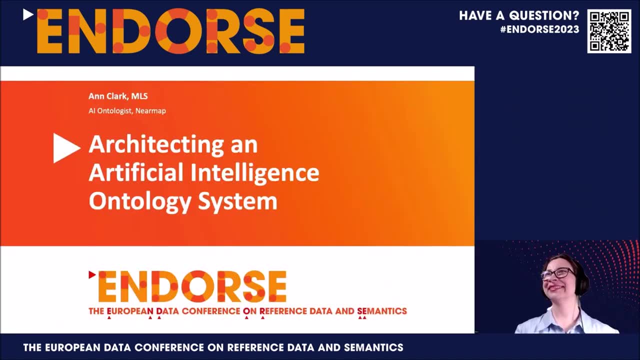 to see your slides and hear your presentation and hopefully have some good questions and conversation at the end. So, Anne, are you there? I am, Yes. you are Great. I can see you. I can see your slides ready to go, so the floor is yours, Wonderful. thank you so much. Well, good morning. 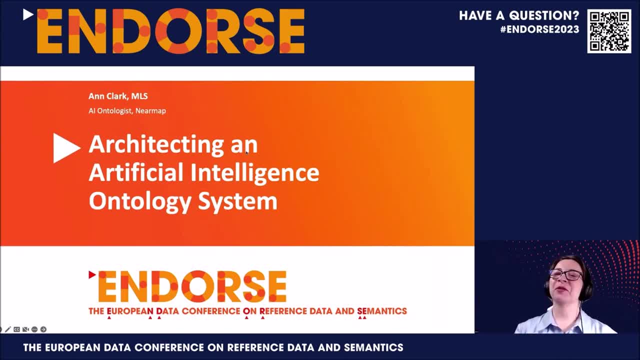 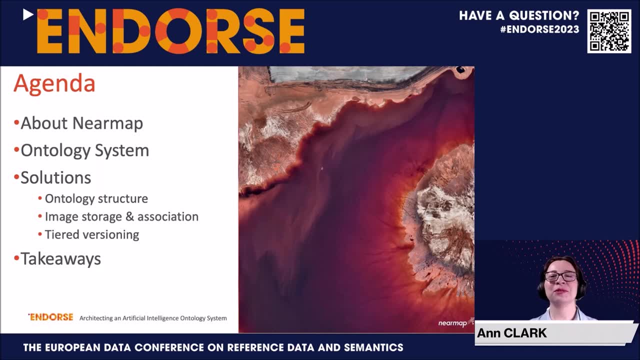 from Sydney, Australia. I'm Anne Clark and I'll be presenting on the work done with my colleague, Zef Yap. So today I'll tell you a little bit about Nearmap, show some system requirements, highlight three feature solutions and discuss key takeaways before taking your questions. 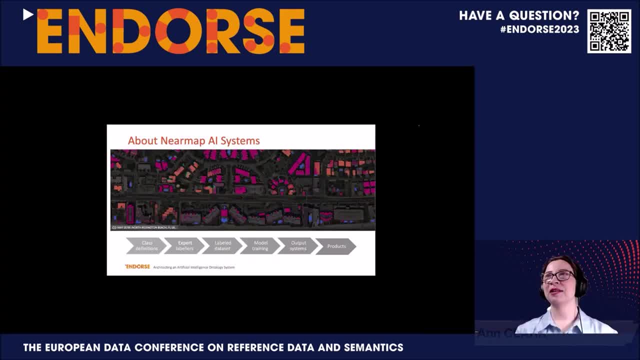 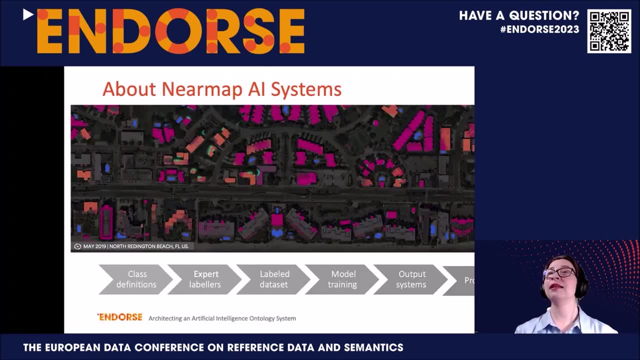 Nearmap is an aerial imagery geospatial intelligence company that uses its own patented computer Camera systems and processing software to capture wide-scale urban areas in the United States, Canada, Australia and New Zealand. Artificial intelligence at Nearmap was launched in 2020.. 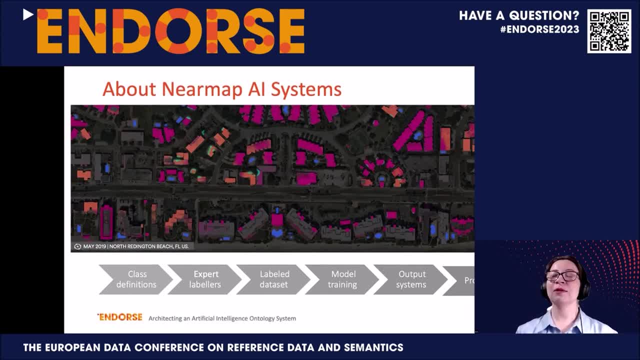 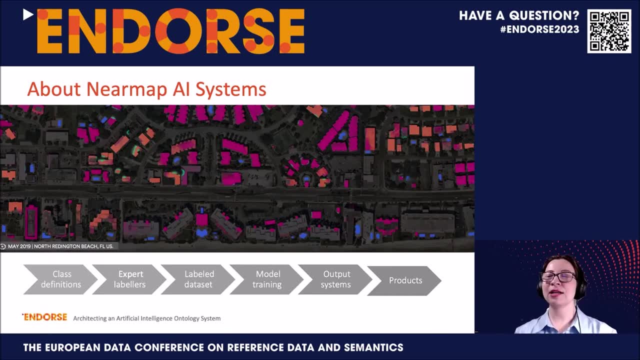 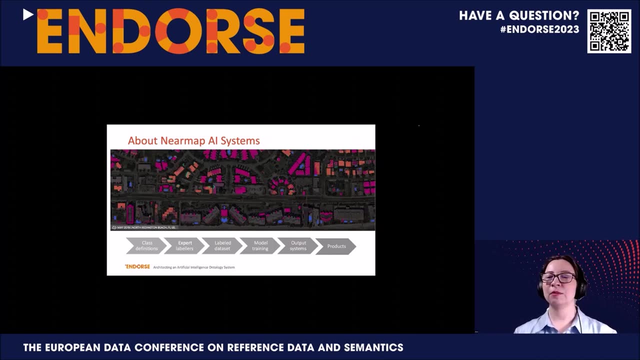 Definitions are the foundation of AI decisions. We rely on expert labelers to manually log class tag classes like buildings, power poles, lawn grass and more. in our imagery, This becomes the labeled data set. Nearmap uses the most advanced machine learning technology: Nearmap 3D 16060.. 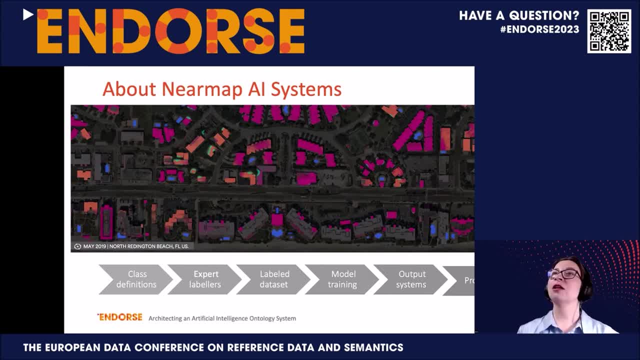 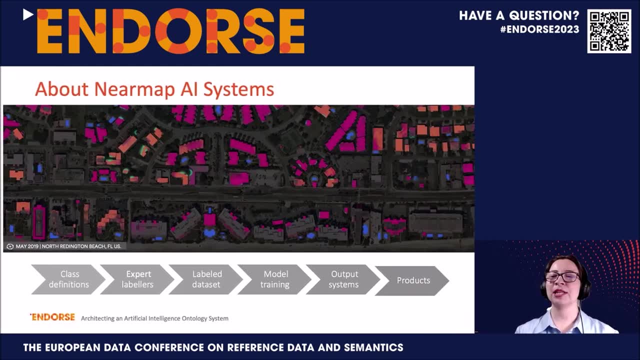 Nearmap is a tool that PlantarASE and Antalya use to train our powerful machine learning model that feeds into industry specific data products. With the ontology, we want to be able to answer questions such as: is a solar hot water system different from a photovoltaic solar panel? 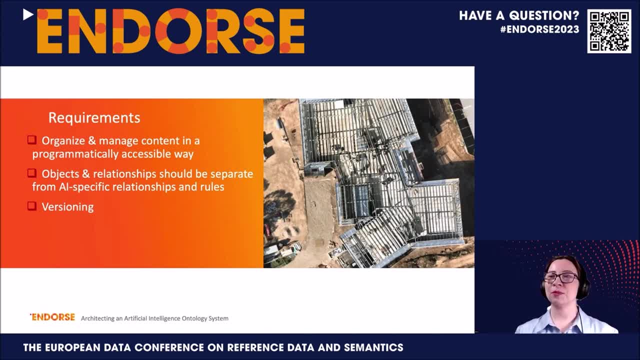 Is that rust or dead leaves on a roof? To answer these questions and more, meant to define and model. When I joined Nearmap, definitions, logic, rules and labeling instructions were managed as text in a Wiki To share with other systems. meant copying and pasting. 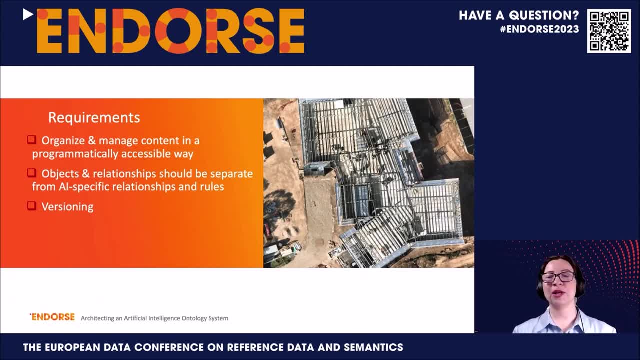 My remit was to design an information management structure to enable leveraging texts and relationship rules in a programmatically accessible way. Logic about physical objects should be separate from logic about AI layers. Ontology scope is not customer or product focused. Class level versioning was essential. 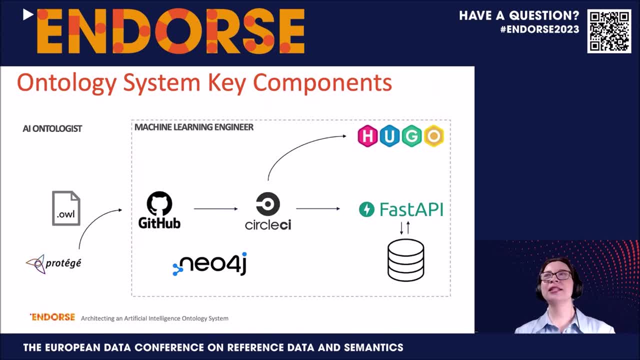 to capture layer changes over time. Our system looks something like this: The ontology gets serialized to an OWL file which we commit to a working Git branch. When we push the commit, a CircleCI job extracts any information we know will be commonly accessed. 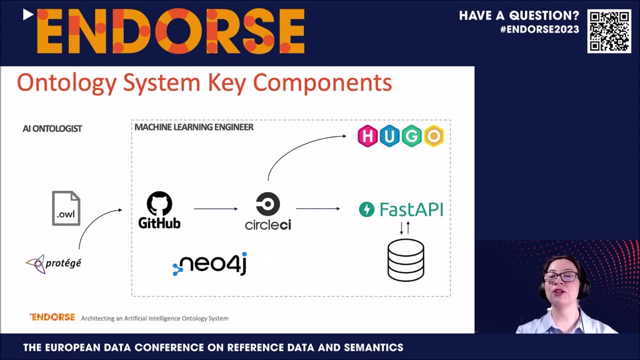 and passes it to our backend API. When the job passes, definitions get published as a static site for consumption by team members and downstream apps. We currently use Neo4j to import RDF XML files without us having to parse them ourselves. Our backlog includes exploring additional visualization. 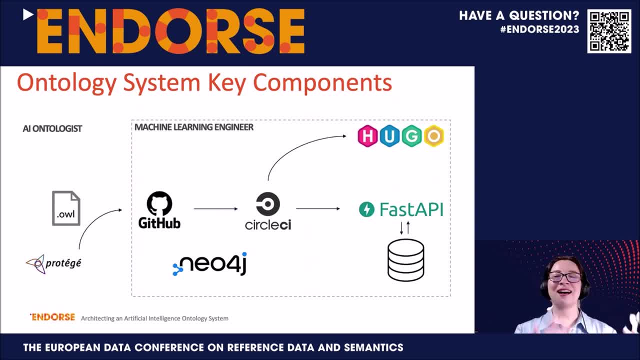 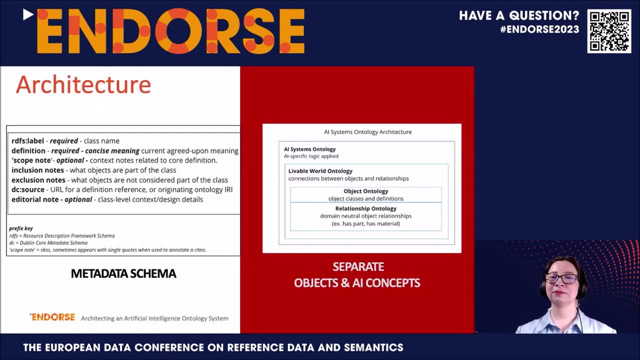 and analytics capabilities. Next, I'll highlight three key system design solutions, architecture, image storage and versioning. Determining what to include as class annotations was one of my significant achievements. I was able to leverage existing ontologies for core concepts such as a label. 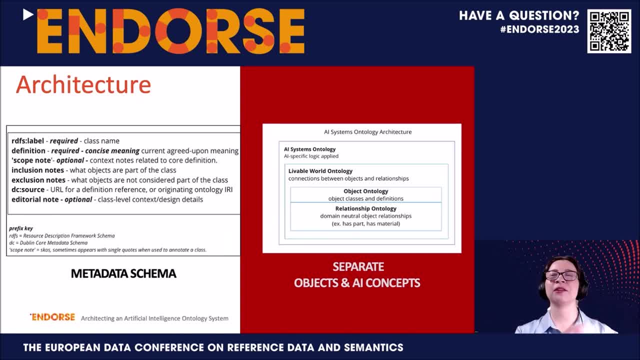 but ended up coming up with my own little schema, as you can see here, cobbled together from both existing and newly created schemas. The ontology is in Australian English and does not currently capture language variants for labels. Localization of classes and descriptions is managed by an in-house design team. 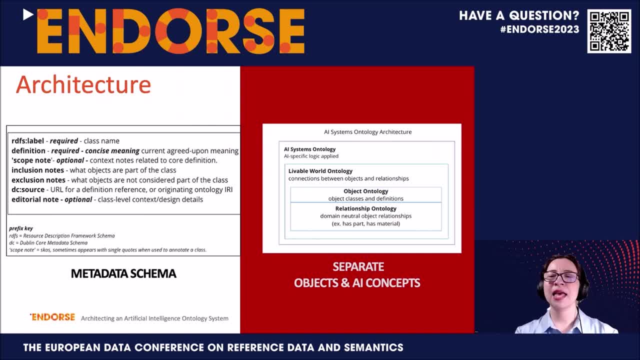 including a technical writer. For example, our Gen5 Alpha class Tyre is spelled T-Y-R-E in the ontology, but customers in the US will see the spelling they're used to, which is T-I-R-E To keep AI and object classes separate. 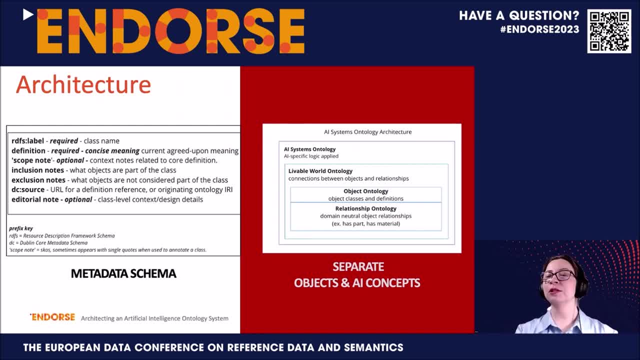 I created separate ontology files. This enables real-world logic and relationships to be applied without the complication of AI concepts. Object and AI classes are related in an overarching AI systems ontology- Again product-focused relationships, AI systems and AI systems, Object-focused relationships or logic such as what version of AI? 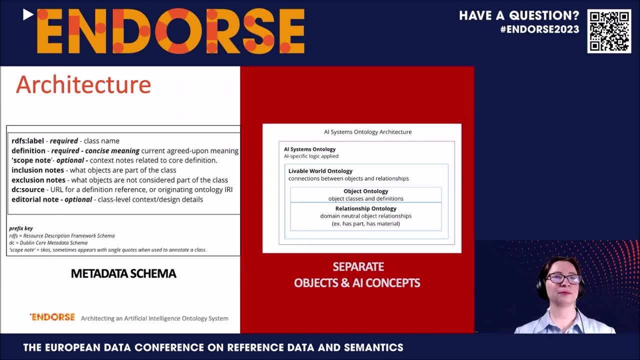 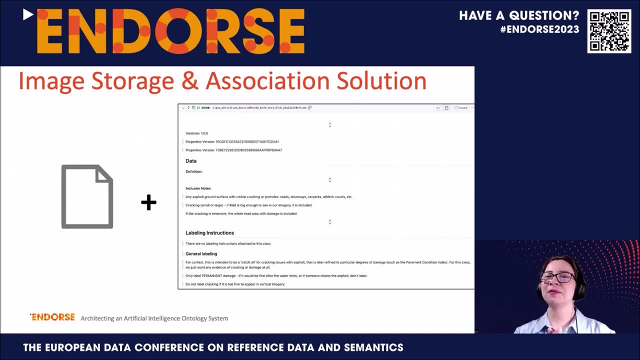 does this class belongs to are not part of the ontology, So next I'll talk about image storage and association. Besides the definition and a label, each class has associated labeling instructions and between 10 to 150 example images. How to document and manage this metadata took a bit of trial. 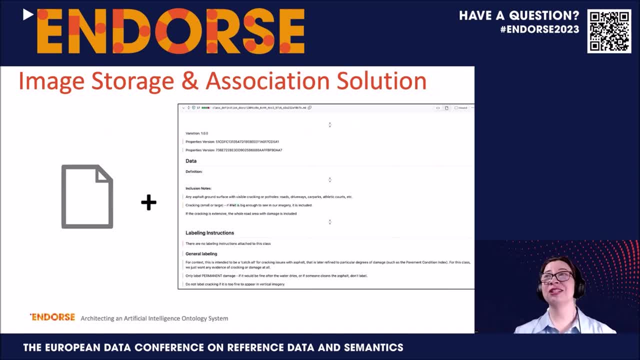 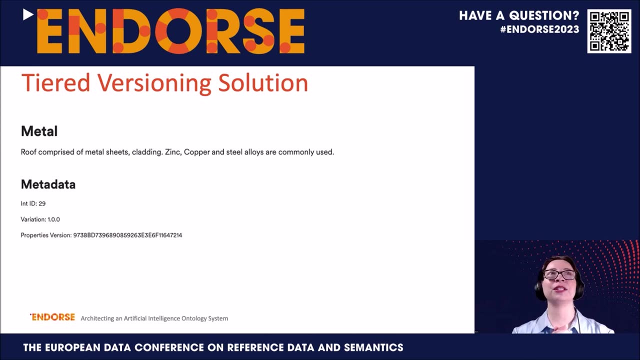 which is a huge step to be able to deliver a high-quality, took a bit of trial and error. ontologies are not databases. therefore, labeling instructions and example images are stored in separate files and associated with the ontology class by uri. which leads me to the third item, which was the tiered versioning solution. 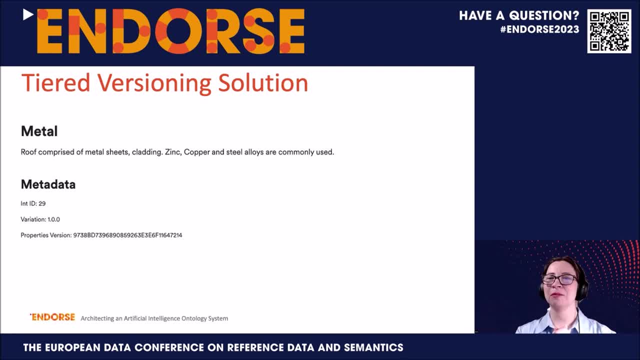 versioning is the area i think we actually got the most requirements around and we ended up segmenting versioning into four separate areas. excuse me, the uri minted by protege identifies the class itself and is what i use in the system, as i said, to connect the class to labeling information and the example images, the integer id. 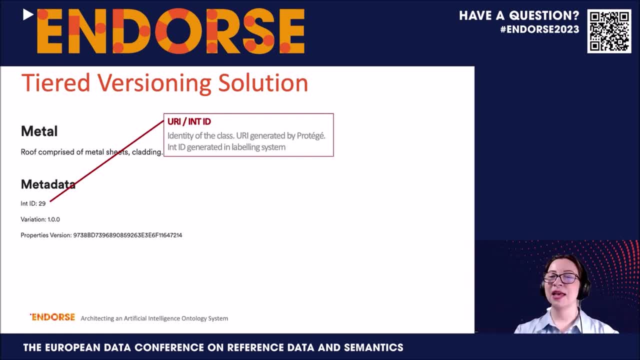 is generated when a class is created in our labeling system and is used by our expert labelers, downstream systems and customer facing content as a unique identifier for the class. any data set breaking change the type of significant. some of the data set breaking changes the type of significant. some of the data set breaking changes. 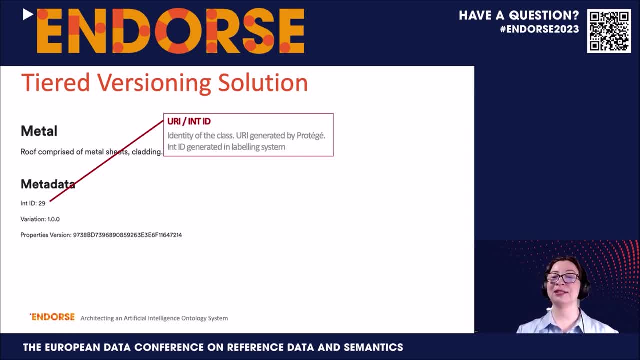 semantic change that would not allow us to continue using existing labeled data for training is considered a new class. this requirement came directly from the labeling team. significant but not data set breaking changes are captured by the variation at the class level. when implementing this structure, we weren't actually sure how useful variation would be. 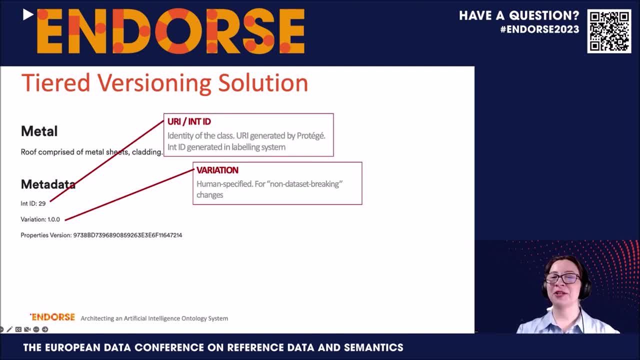 but a few weeks ago i actually needed to use variation to update a developing class and i was really glad that we had included such granularity in our system. we generate a properties version of class data to fulfill audit and traceability needs for downstream system teams. this excludes all example images or labeling instructions. 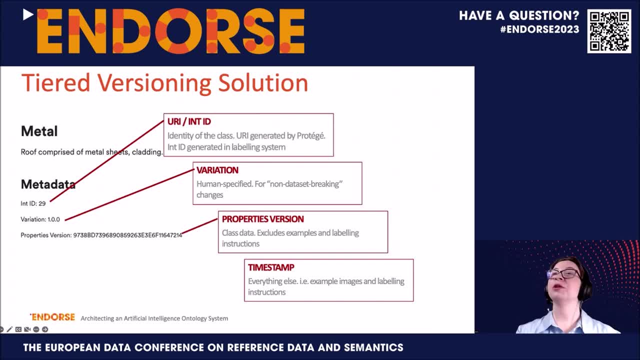 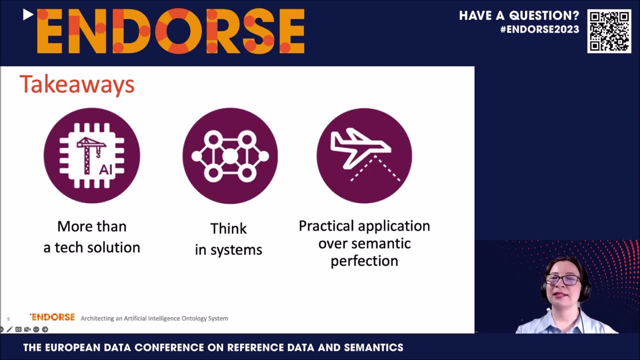 we track image and label instructions, changes with system timestamps. one early lesson learned was that not all pain points or challenges about language management can be solved by technology, such as quality control over all your all of your metadata fields completed or how to define a new class. what you don't see in the system architecture solution is the proposal process i designed and 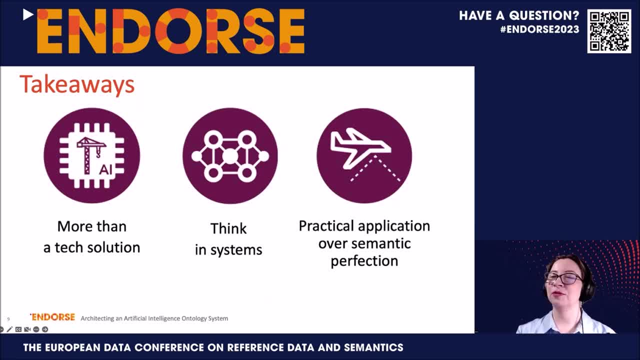 implemented and to use to develop generation 6 ai classes. secondly, about thinking in systems. to create a programmatically accessible system and make it a trusted source of truth required full ai team collaboration and designing with connectivity in mind. this is one reason we have more versioning tiers. ontology system content integrates directly into our in-house labeling tool. 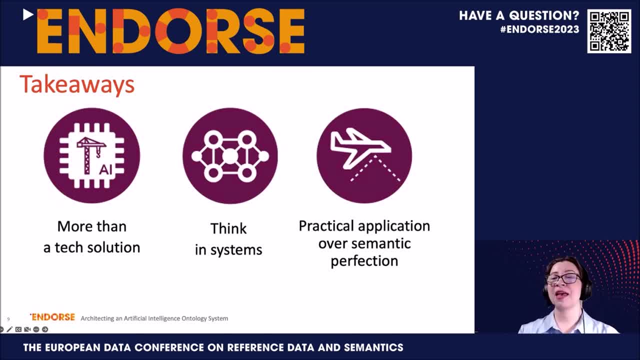 ensuring our labelers have the latest information while working on a job, so this means no more copying or pasting. we have additional internal systems to integrate with and some logic focused backlog items, which leads to my third point. i could have spent years testing and teasing out the nuance of each class and modeling relationships between them, 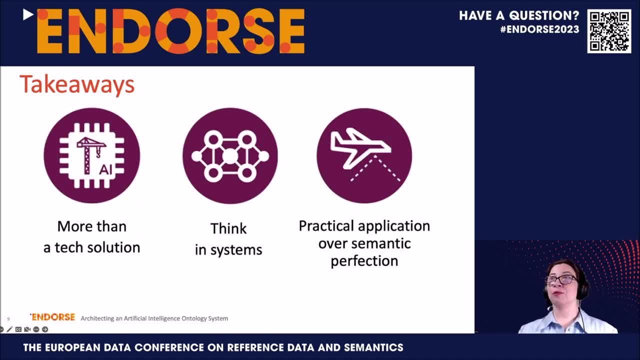 but then we wouldn't have a working or usable ontology system right now. instead, i limited ontology scope to a set of 16 reusable relationships. we got the system itself in place and in use and plan to continue evaluating relationships based on team requirements. so with that i thank you and look forward to any questions. 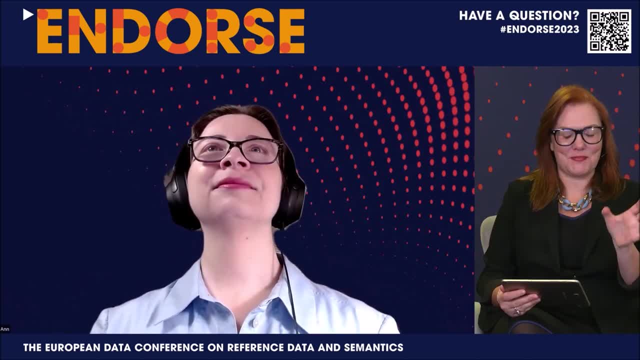 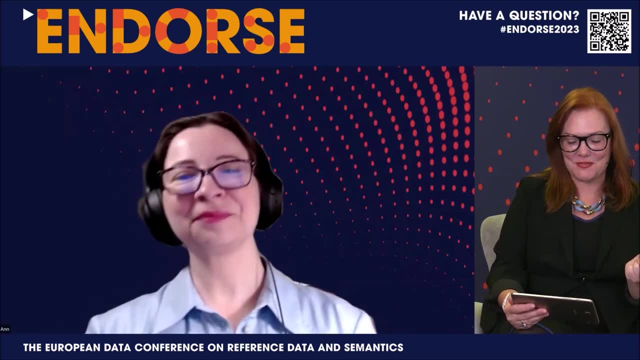 thank you very much, ann. that was a lovely guided tour. i appreciate the slides. it was very easy to follow, especially at this point of the day when i know people have taken in a lot of information, so that is much appreciated by myself and, i'm sure, our audience as well. we do have questions, however. 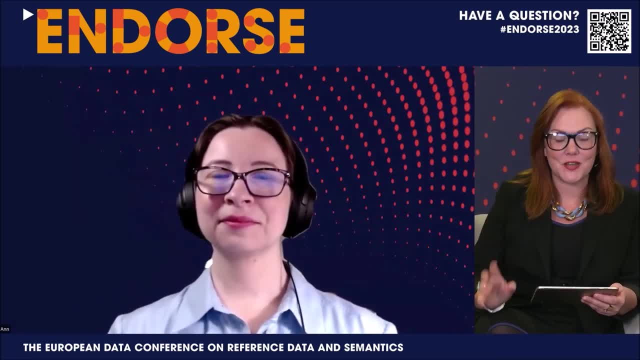 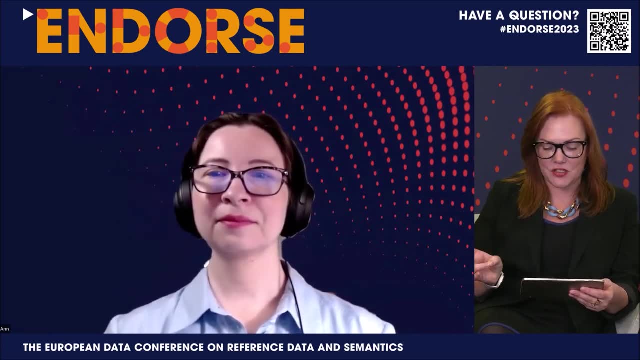 just for, uh, for you, just to elaborate a bit more on some of the topics you raised. so one question is asking: could you explain what are the challenges of the new system and how do you deal with them? what are the artificial intelligence, specific relationships and rules and how they differ from? 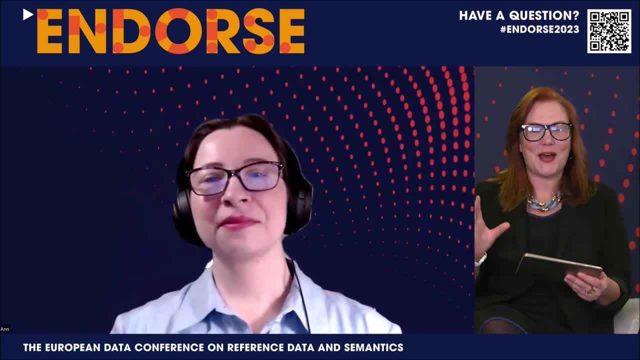 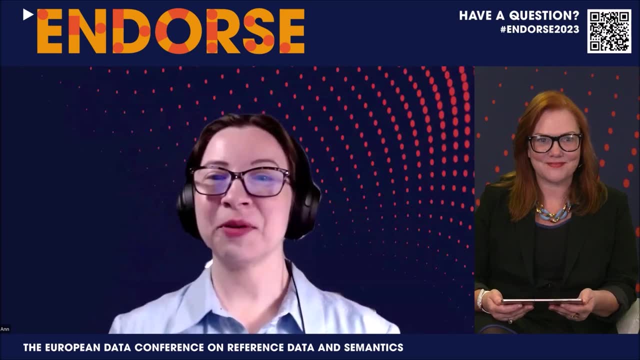 objects and their relationships. uh, you know, feel free to expand on that, because i think that is something that a couple of people also picked up on, that they want to know more about. that's a great question. um, so, for example, some ai relationships are. is the class line of sight? 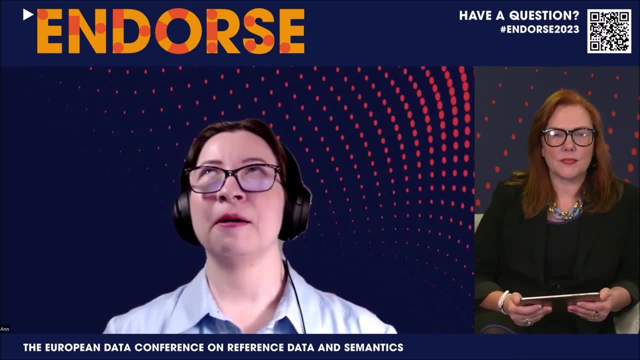 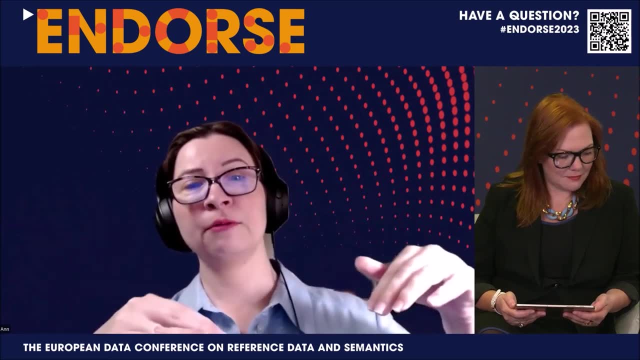 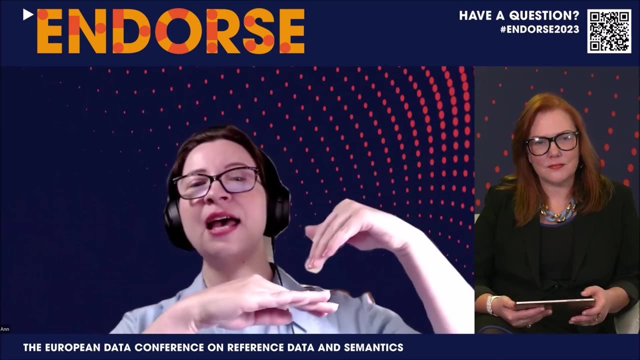 or non-line of sight. and that's: if, if um imagine you're looking from the air down a building or tree, can you see through the tree to what's on the ground, or do you not see through the tree? and the tree is literally your line of sight. does it block anything below it? and that has some 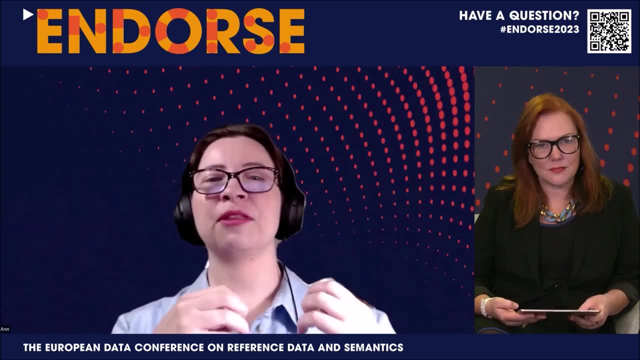 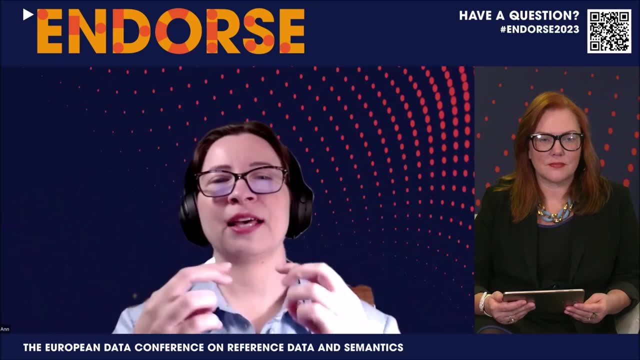 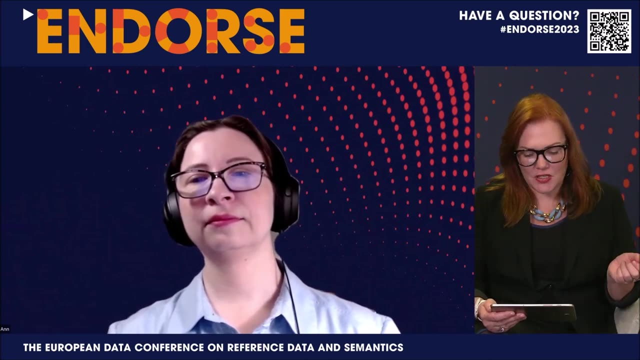 implications for how our model works and for how we label. but we thought that that kind of information, of relationships would clutter what things are in the real world. so we decided to keep a separate ontology for those kinds of relationships. and in which way do artificial intelligence, specific relationships and rules allow machines to enhance the capabilities of? 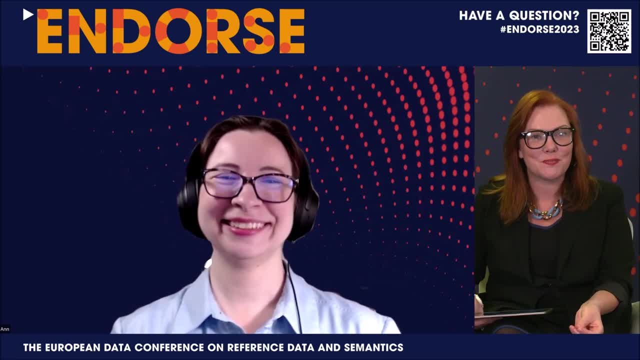 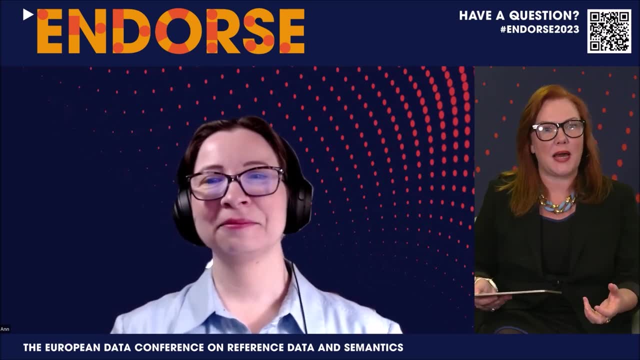 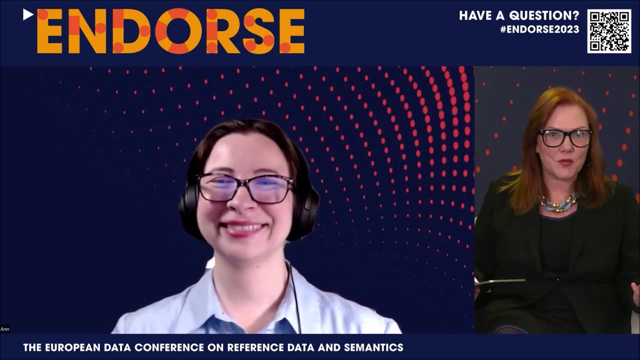 the human mind. this is a topic that has come up a few times with previous speakers. it's obviously something we're going to talk about at indoors conference every year. but where do we find that nice balance? how do we get the ai to work together with the, with the human linguists and ontologists, so that we get the best of both? 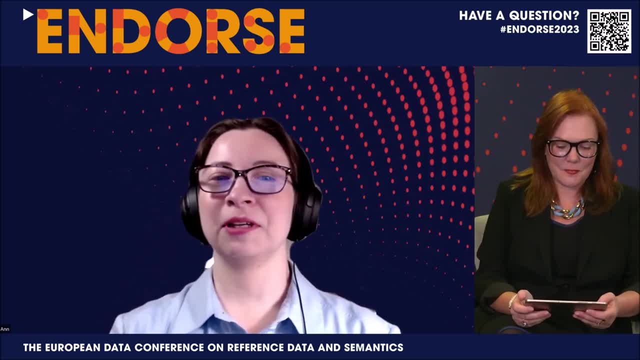 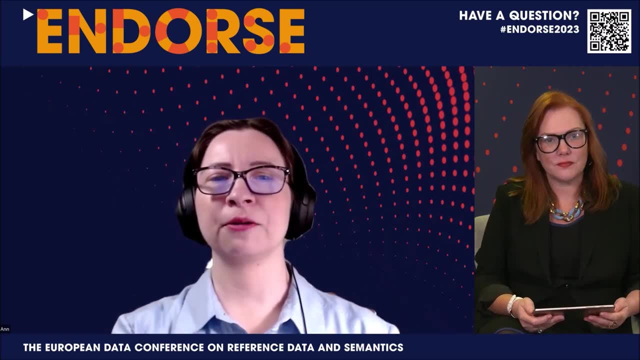 worlds. that's actually where we're looking at a lot of things right now. what i started with the ontology was building out layers we had already created, so we have about 78 layers that are currently available to the public and about 150 total in the background and, as i said before, i 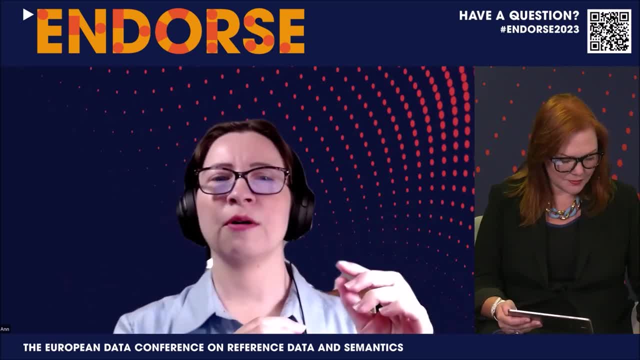 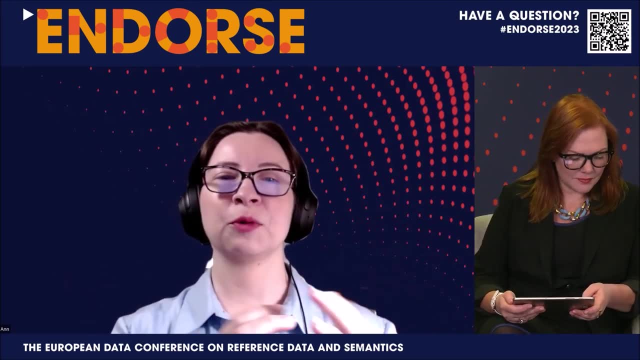 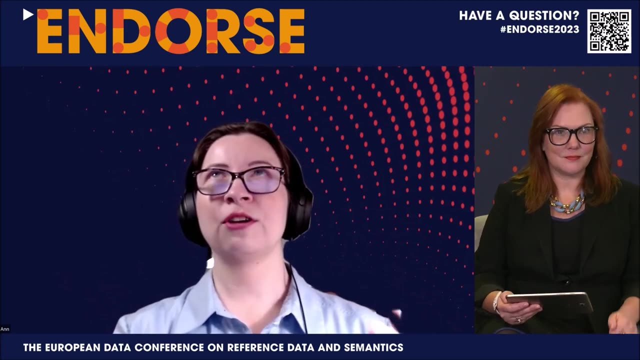 need logic, so subclass, superclass, or type of roof material or type of vegetation height. those kinds of items were only written as text, and so what i'm working with the data scientists now is to actually identify what of those logic statements can we use as rules that they can then use to help. 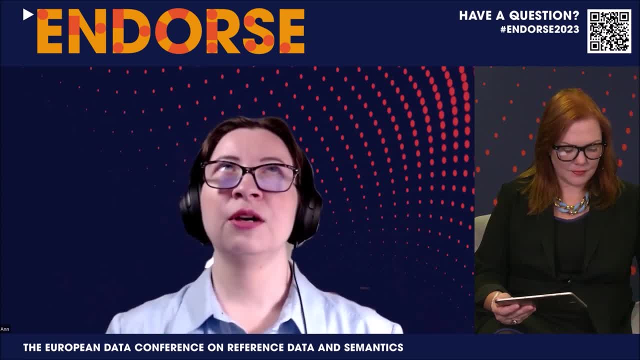 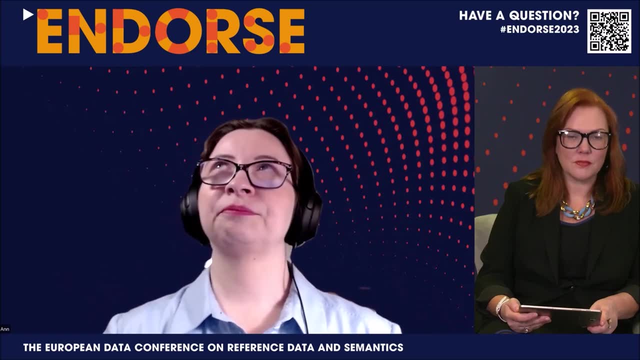 tweak their models a bit. the question i asked in the beginning was: you know, can you tell rust on a roof versus dead or dry leaves? and so one rule we have is that rust can only happen on a metal roof. so if the roof isn't metal, you already know. 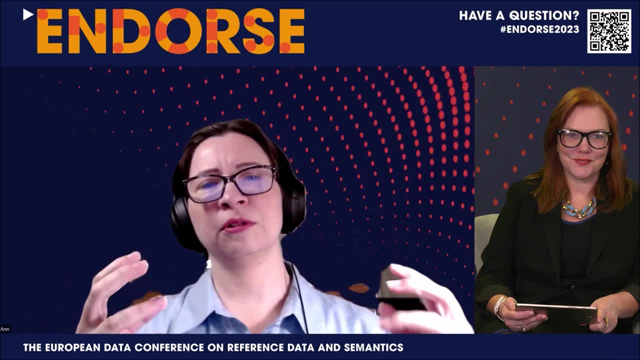 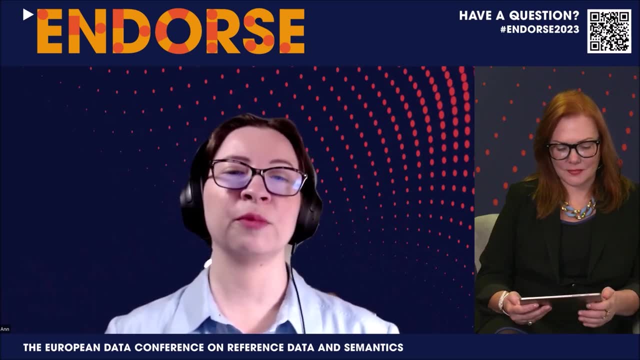 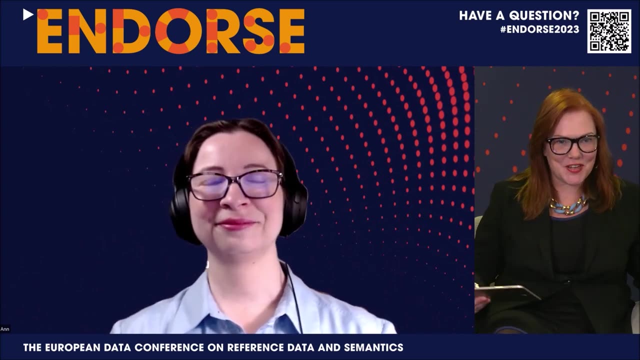 that it's not rust, and so that's a simple rule about the physical properties of something that we can implement, and it can be used to help train the model to make it give better predictions. um, and because again, we have all. we've so many, uh, public policy experts and public administration. 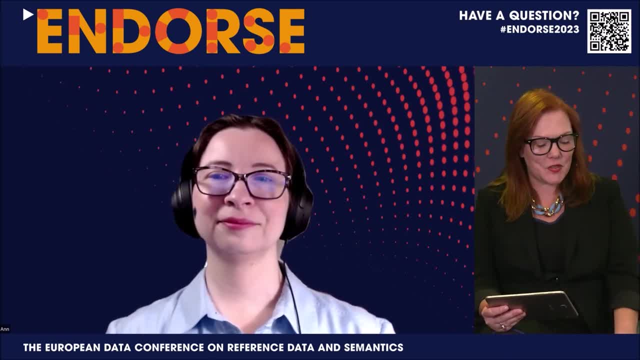 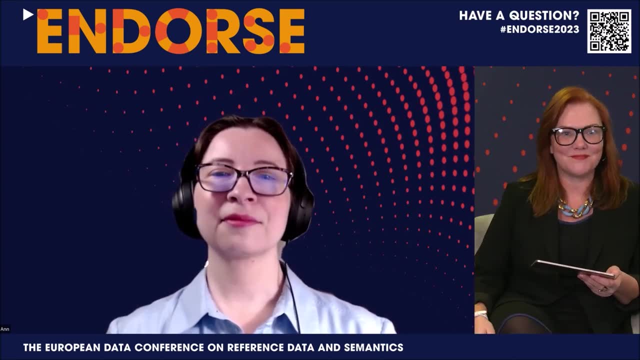 experts here. can you give us some examples of where you might see this used in public administration or how that might develop jobs in the future in that area? a lot of our current customers use these things, especially during the pandemic when they couldn't go out to sites. 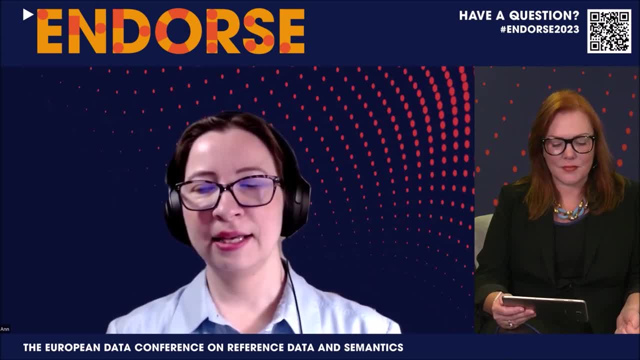 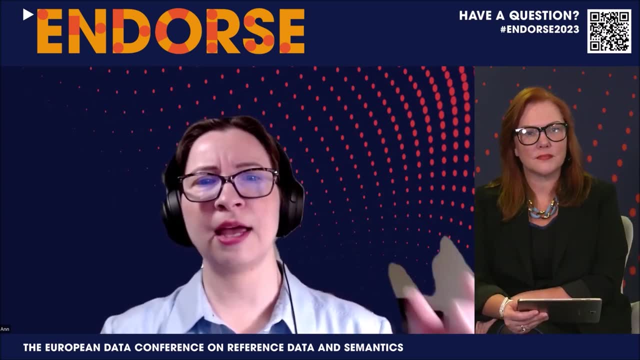 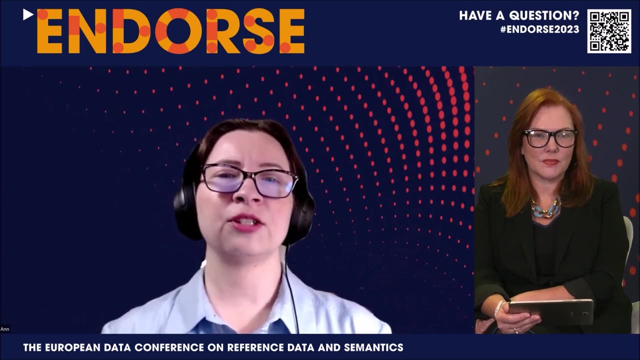 so a lot of our, a lot of our customers are using it as a site evaluation tool, and so i see the competencies needed for identifying content through ai results versus actually going out to a physical site is a little bit of a shift in linking. it can also be a good thing for safety, where if someone